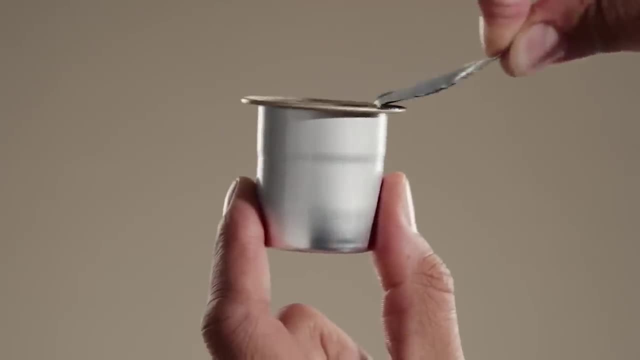 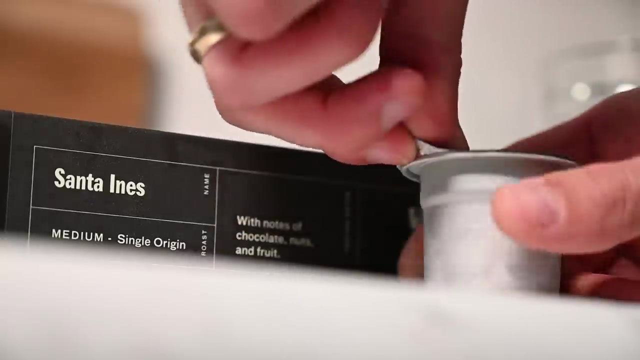 calibrated to extract as much flavor as possible from the beans, Which is then flash frozen into what they call an icy puck- I don't know if I've ever heard a cooler name, And all I do- since I drink my coffee black- is I drop the puck into my cup, pour in my hot. 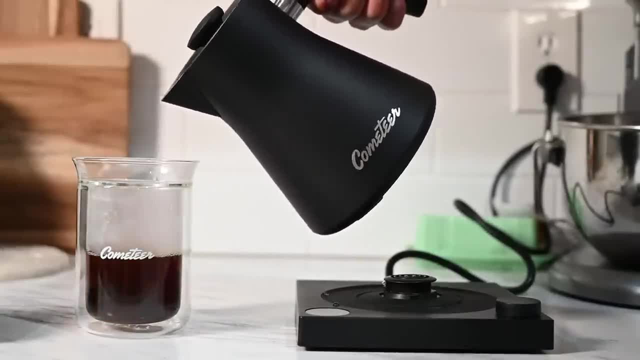 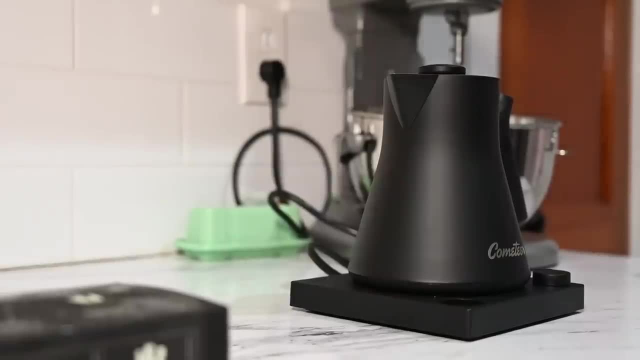 water that melts the puck, which, by the way, is brewed 10 times stronger. so I can do just this. it's not diluting by any means and I enjoy it- By far the best cup of coffee I've ever had. And this fully recyclable, as is all of their packaging and shipping materials, which for 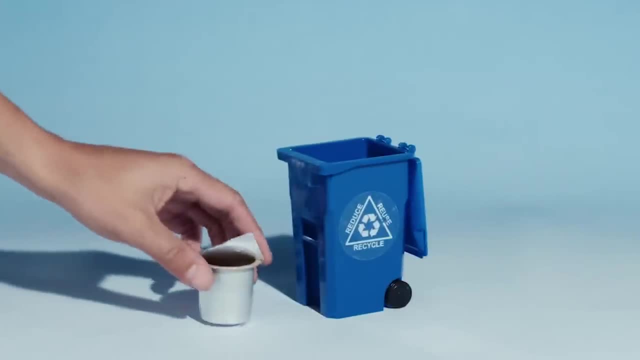 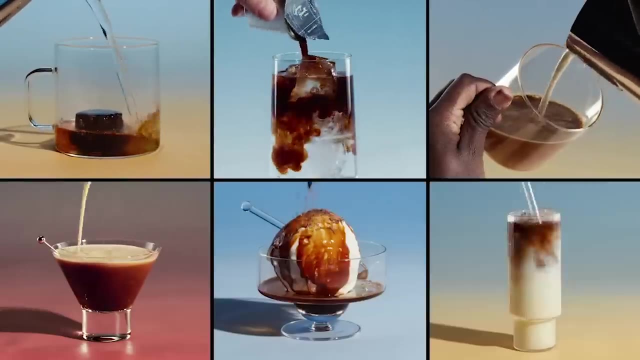 someone living on the coast. seeing trash washed up onto the beach left and right is incredibly important to me. Speaking of which, I've been taking this on our beach days. I've been taking this on our boat days. I just put a capsule in my bag and once it melts, I just pour it over. 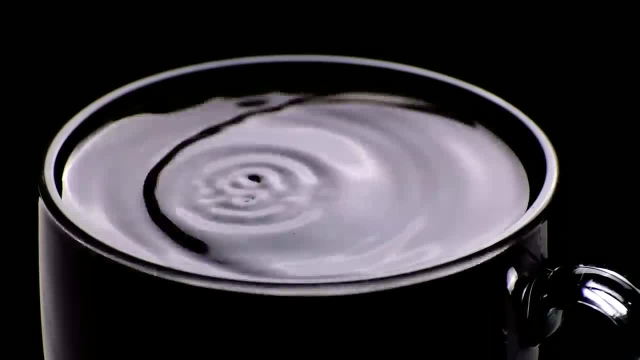 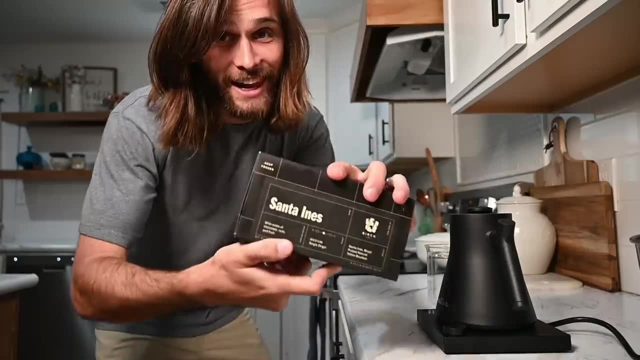 my ice water. And don't tell because while I almost always drink my coffee black, sometimes instead of water I'll pour it over iced milk to make myself a latte If you haven't tried that, it's really good. 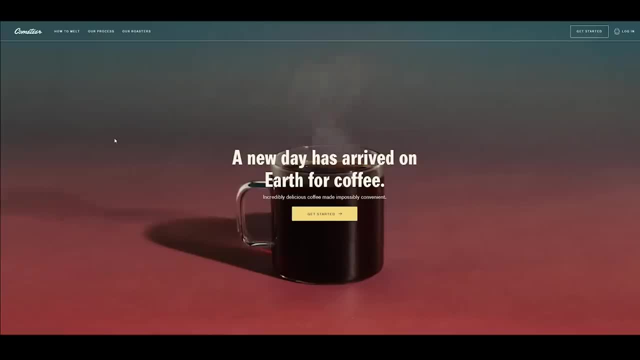 So I'm going to enjoy my coffee and wanted to let you know that currently Cometeer isn't fully open to the public just yet, but by going through my link below you're able to bypass the waitlist and all services. 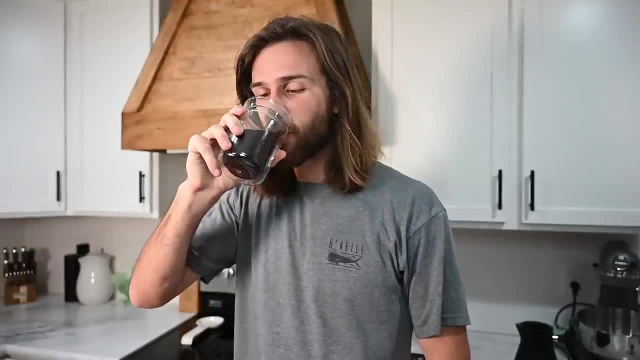 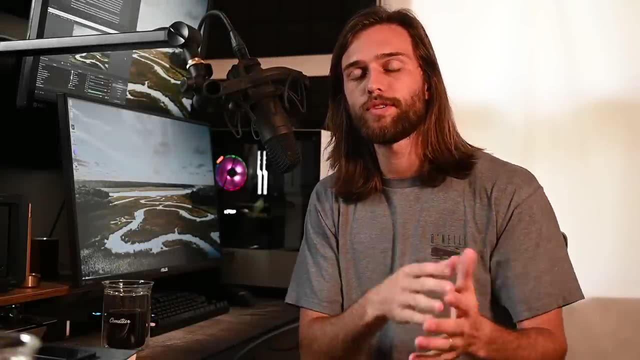 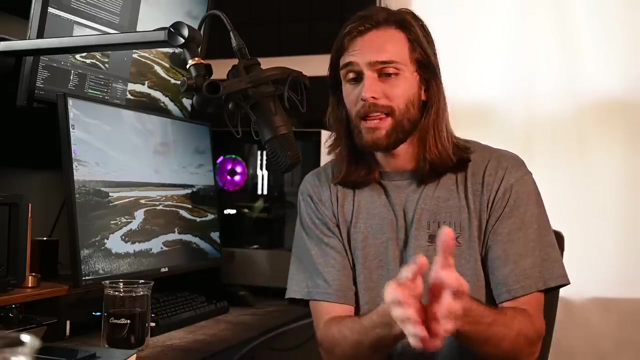 You'll also receive 50% off your first purchase. That's just $1 a cup. enjoy. Most of the experiences you see are from software engineers on YouTube sharing their day, but that is a biased point of view. They're entertainers. they want you to watch the entire video. think about it. 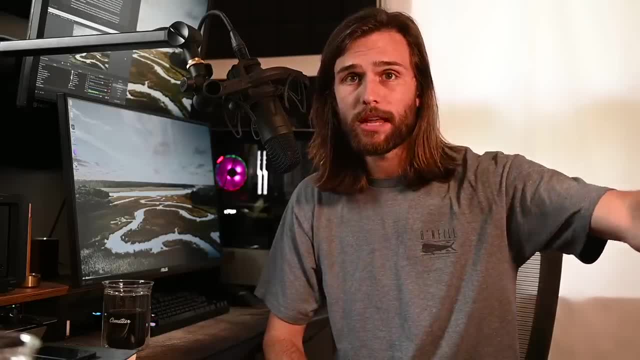 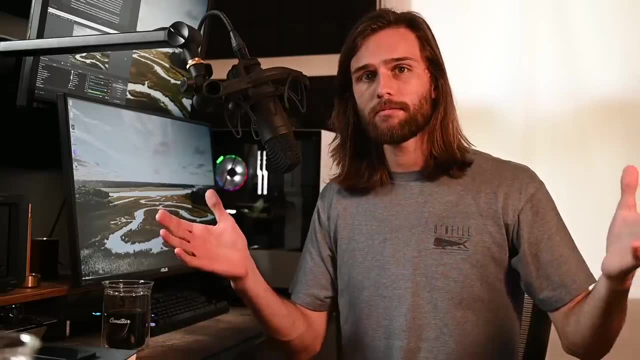 It is a lot easier to sit down and watch an hour long movie that has been directed and filmed and has a story throughout, rather than sitting down and watching an hour long lecture. Can we agree on that? And people who want to share their experience want you to be captivated by their day. 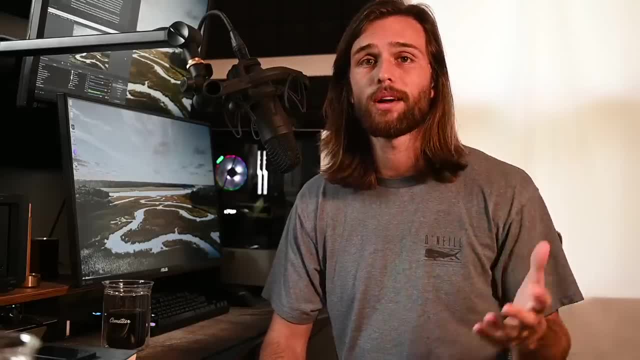 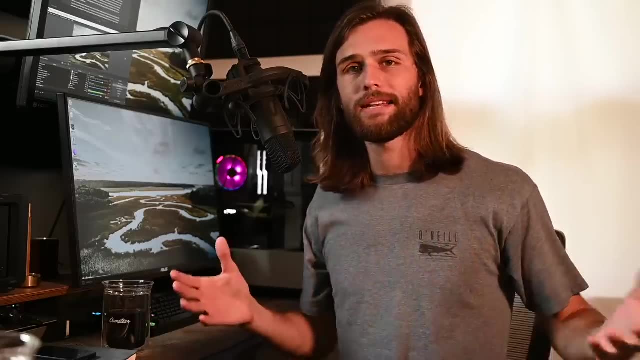 They want you to watch the video, as long as they can get you to watch the video, Because the whole idea with a lot of these channels, especially on YouTube, whether it be software engineer or not, the whole idea is for them or for you to forget about the. 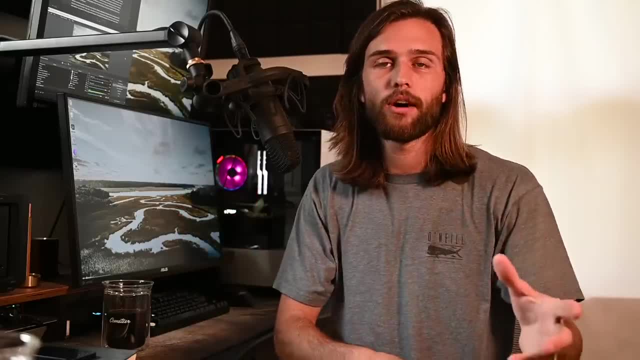 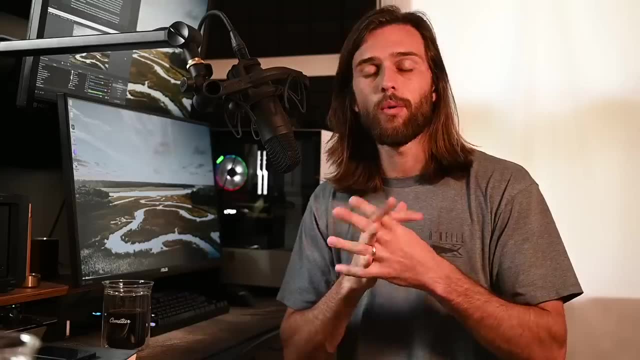 entire outside world and focus on their video, watch their video in its entirety, be consumed by it, be entertained by it. And well, that is the main goal. Whether it is Helping you out or educating you, That is the goal. 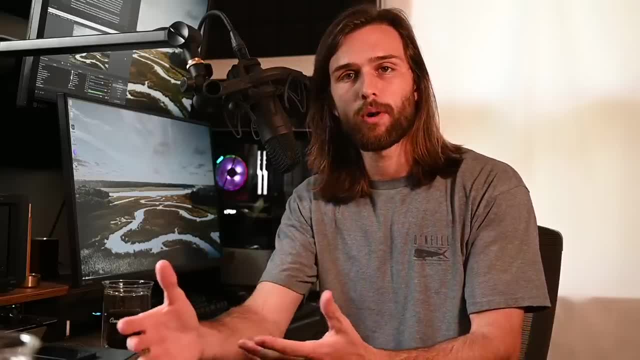 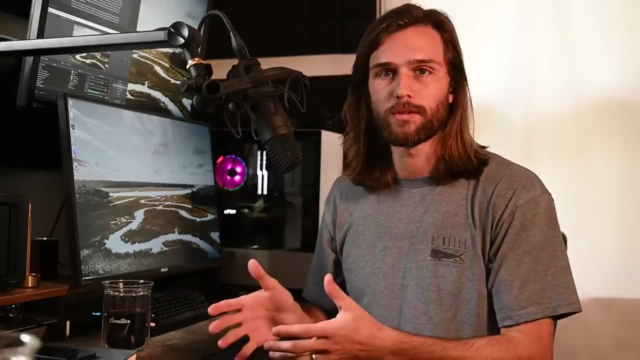 I only bring this up because it's a highlight reel at best or misinforming you at worst. So don't look at these videos and think that's exactly how it is, because you can't see into the minds of these individuals. They aren't just typing aimlessly on a keyboard. 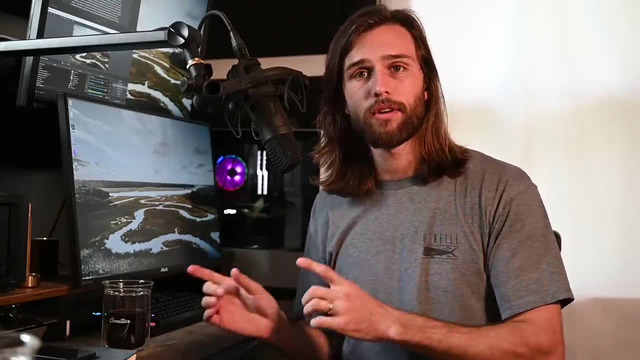 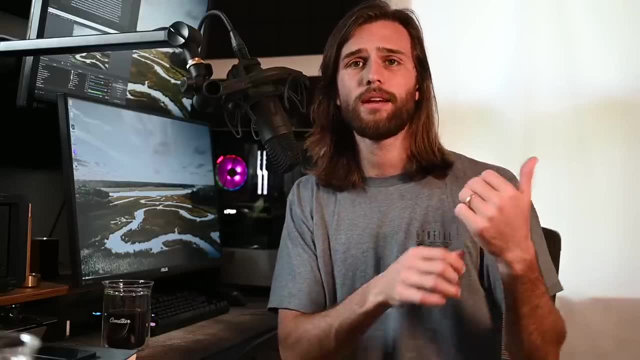 They're deep in thought, trying to figure out the solution to the task at hand and then doing research and implementing that solution in code and in their meetings. they're not just shooting the breeze with the coworkers, they're being told that the entire week's 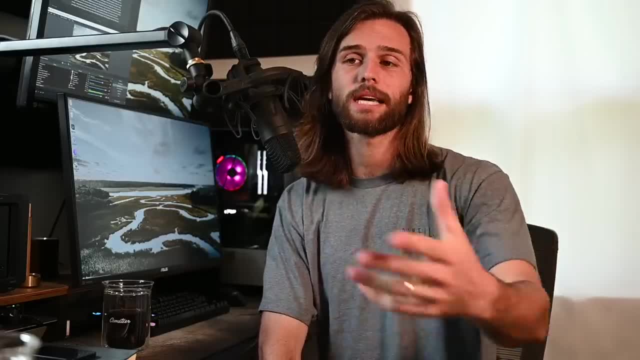 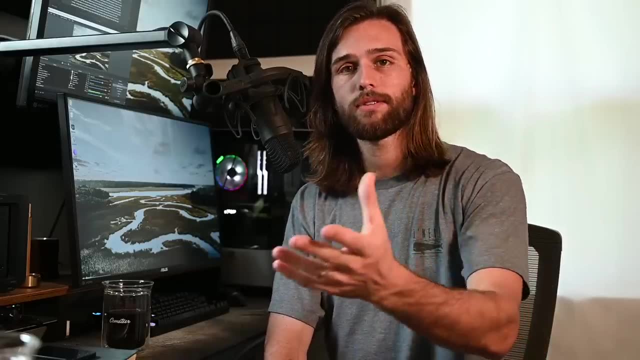 worth of work before It's completely worthless because the client decided to go another route and they don't want that feature implemented anymore, or you're being told that your task was done incorrectly So now you have to redo it, And those meetings are never fun. but you know it's not all bad. 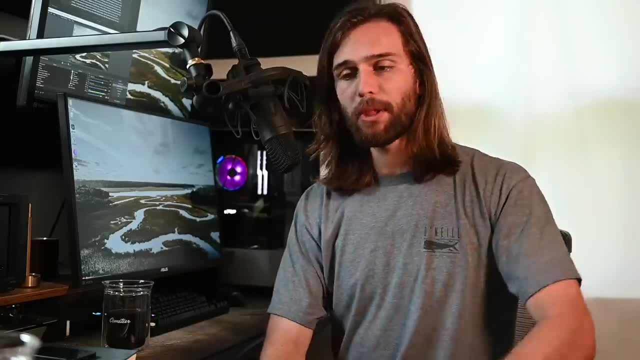 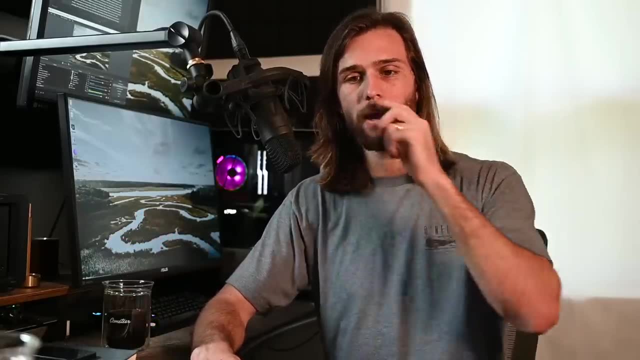 Sometimes you are just shooting the breeze with the coworkers and discussing what to do next, And plenty of the things that I mentioned in this video may be seen as seen as negative or whatever it may be, or it may appear that I'm trying to discourage some individuals. 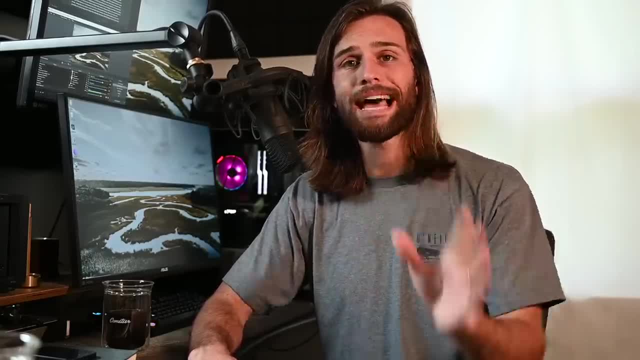 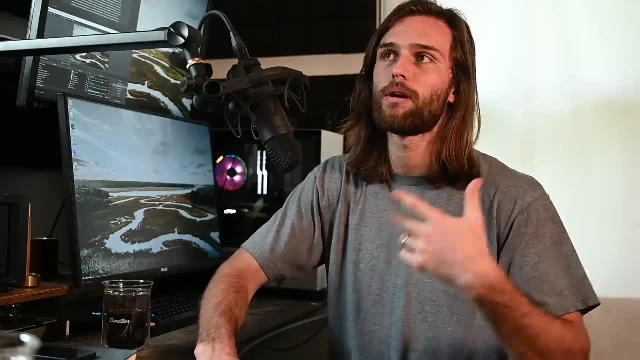 from becoming software engineers. No, I'm trying to show you the reality of what it's like to be a software engineer, not just the good thing. So if I do focus on things that are a little bit more negative, don't see that the majority 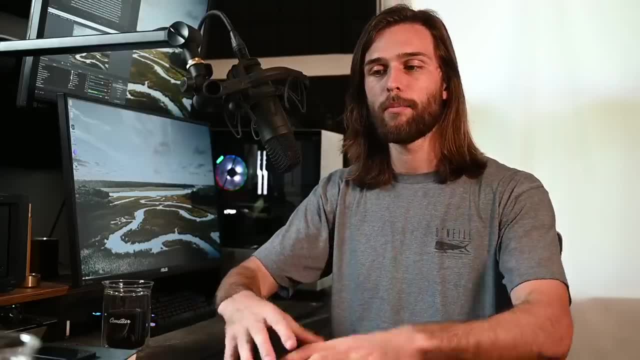 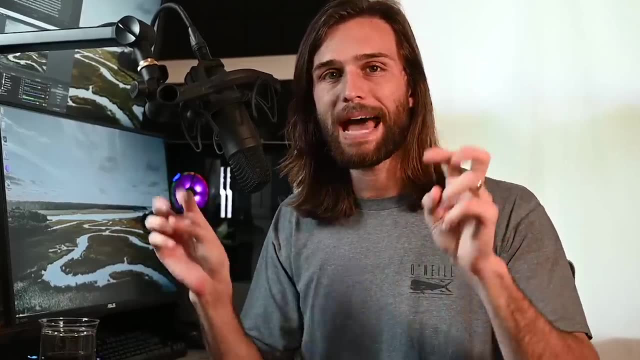 of the job is negative. I'm just trying to counteract all of the positive and all of the good things, the highlight reel that people are putting out there, but neglecting to do so for the bad thing, Because you need to understand that in any job, especially this job, there's a give and 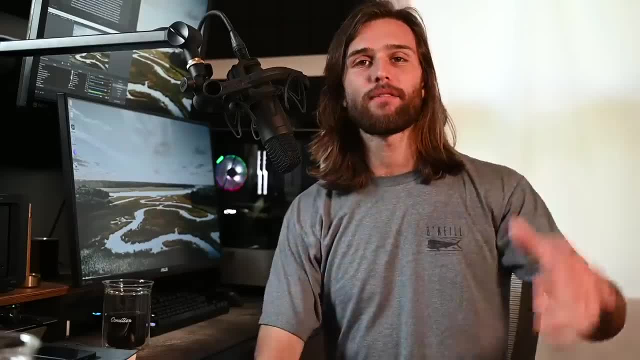 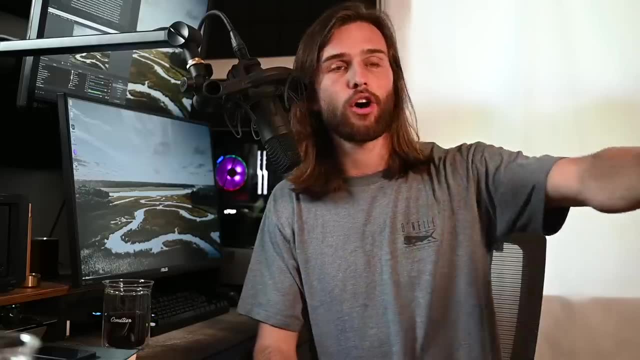 a take, Good and bad, Which brings us to the everlasting question, especially staying on topic, when it comes to software engineering YouTubers like myself. I'm not, I'm not, I'm not calling anyone out in particular. I am a software engineer and computer science YouTuber, just like everyone else. 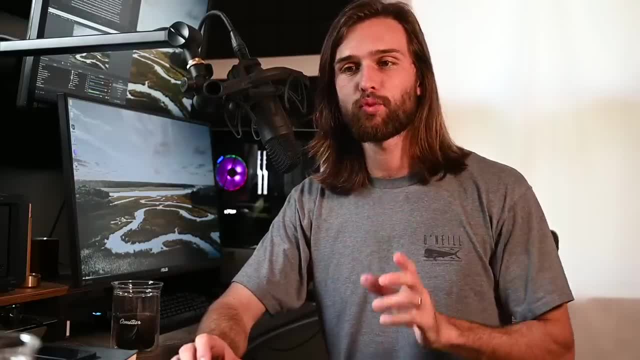 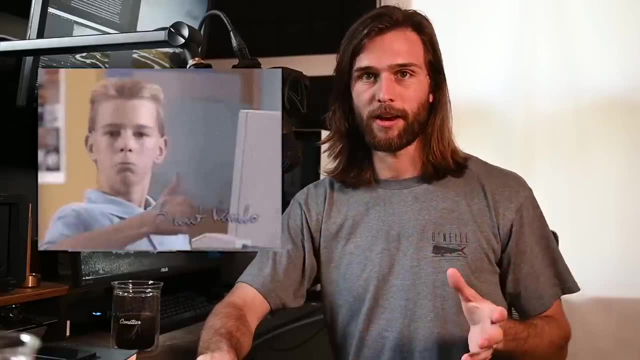 And I made the same videos, because the everlasting question really contradicts how a lot of these people portrayed their day as being always good, always positive, always fun, But most of these YouTubers who display it like that end up quitting their full-time. 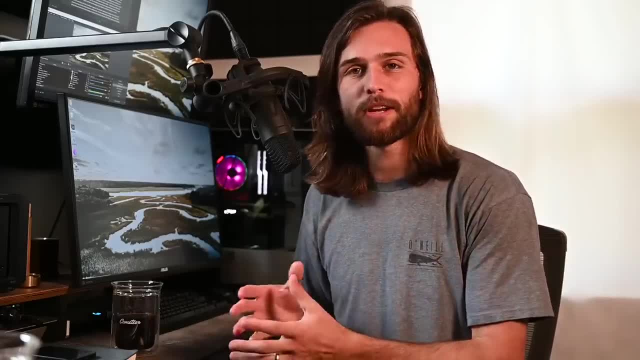 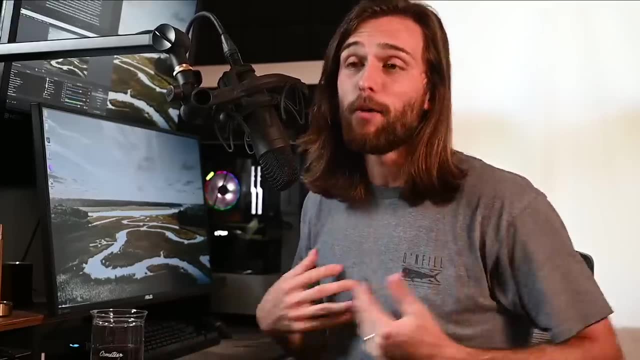 software engineering job to do YouTube full-time. Well, if it is all butterflies and rainbows on the software engineering side of that, then why do they quit that job? I know why I've done it, But for me it may be a little bit different than most. 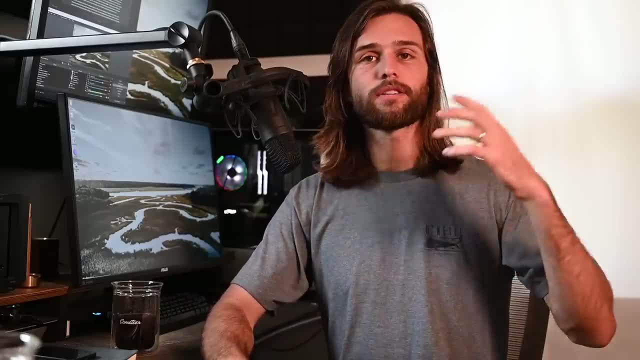 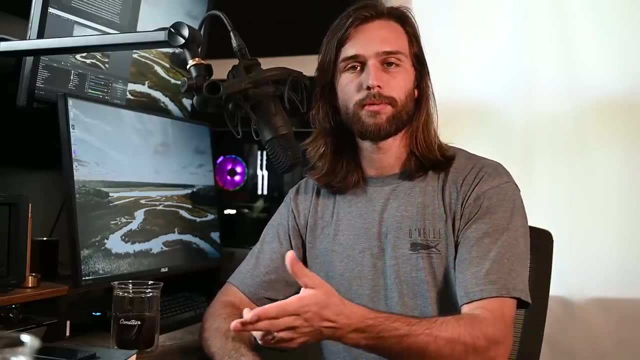 So I've always wanted to work for myself. If I never discovered YouTube, I'd probably be freelancing, So for me it wasn't always about what I was doing, as long as I could do something that I enjoyed and work for myself. 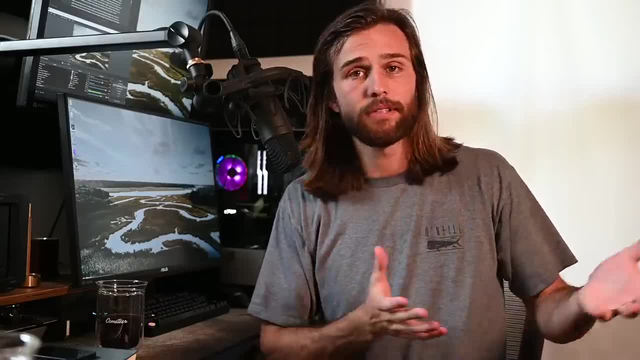 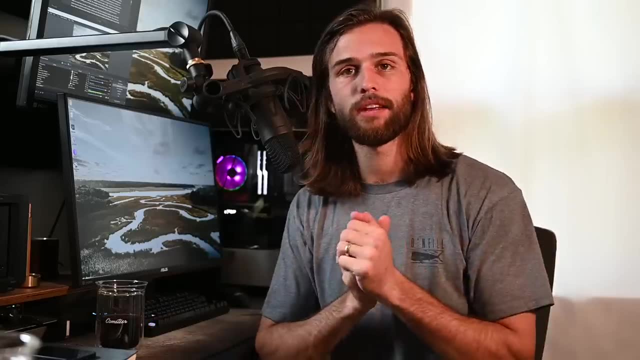 Many of these, Many of these individuals probably shared the same sentiment. After all, they did start a YouTube channel for a reason. That reason could be because they thought it was fun, because they wanted to help people out, or because they saw it leading to their financial freedom. 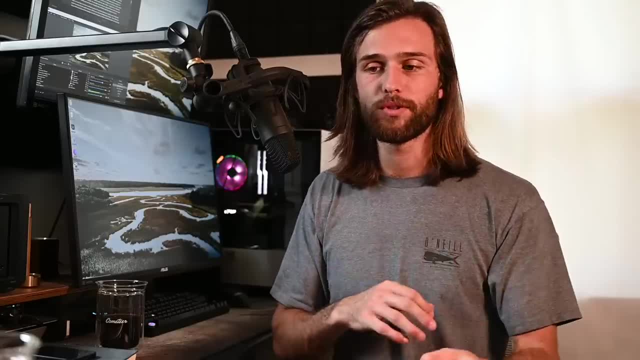 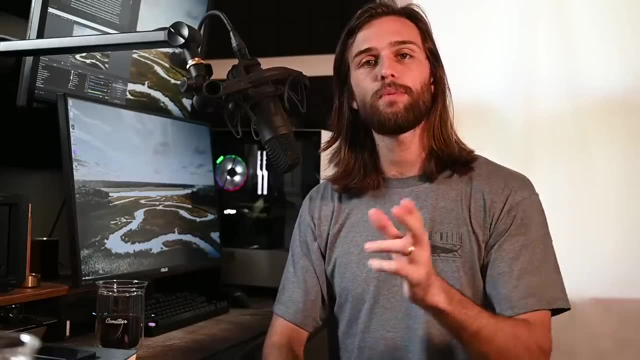 Whatever it may be, they saw this as being part of their future, But also because, if they truly enjoyed coding, this was a way for them to make a living but also be able to work on their own projects. Which brings me to one of the biggest points of this video, which I feel like people never 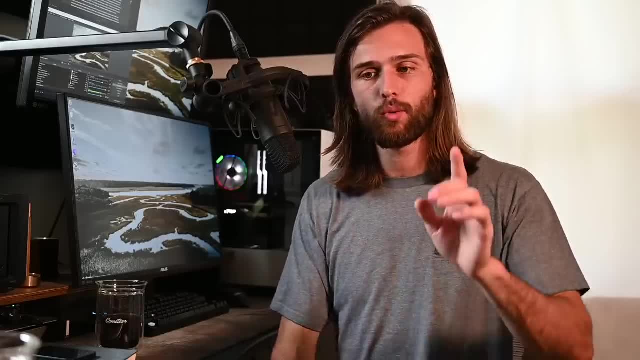 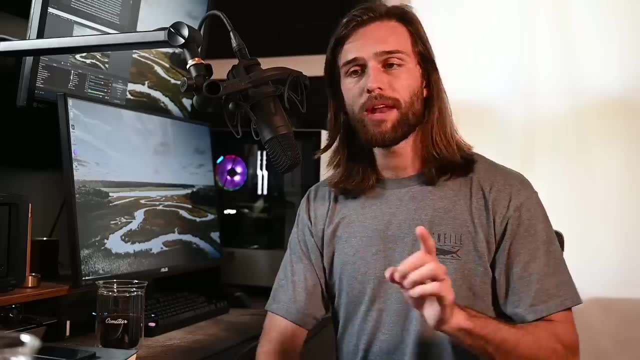 talk about. That is The final software engineer is working for someone else's company, Working on someone else's idea. You may love the idea, you may love working on that app, but you never have the final say on what features are implemented, or even exactly how it looks or the overall growth. 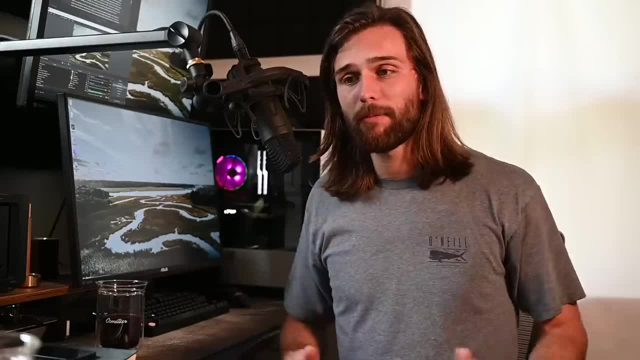 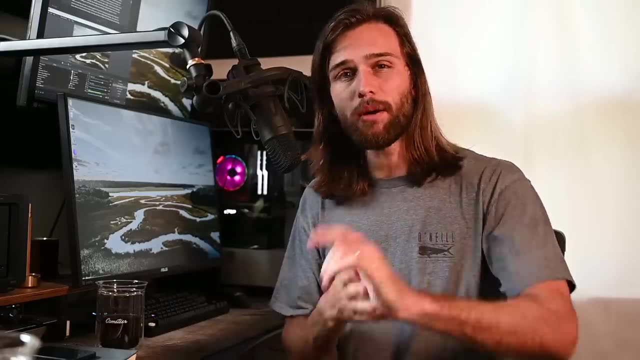 of the company and where that app will be in five years, For lack of a better term. you're very much a code monkey, being told what to do and how to do it with very little creative freedom. Some creative freedom, but very little. 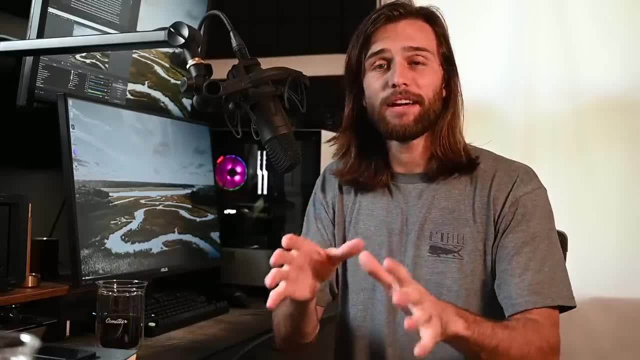 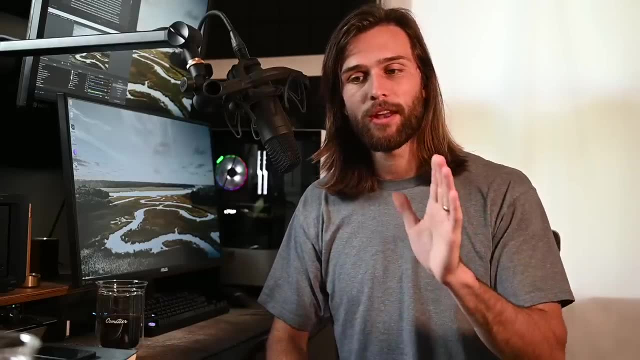 I personally can't work that way, But That may be their cup of tea. You need that direction, You need that structure, So this may be perfect for you. I know people who thrive on not completing the overall idea or worrying about the overall. 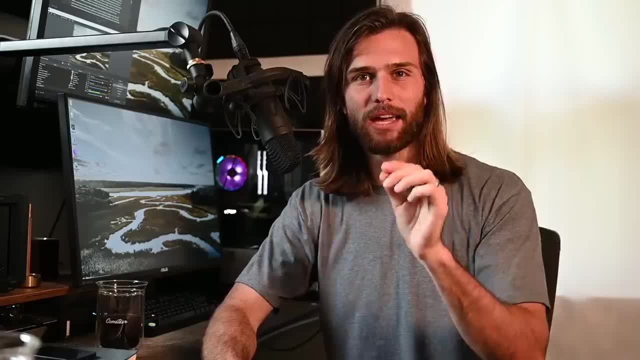 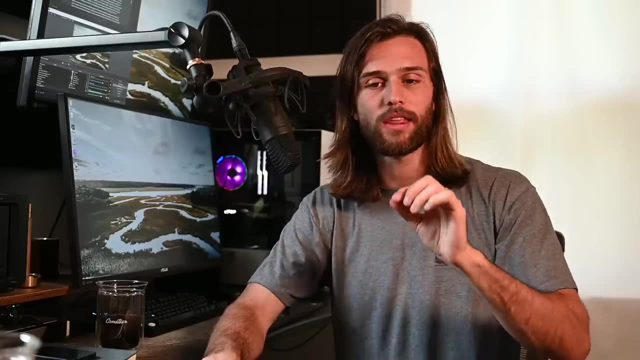 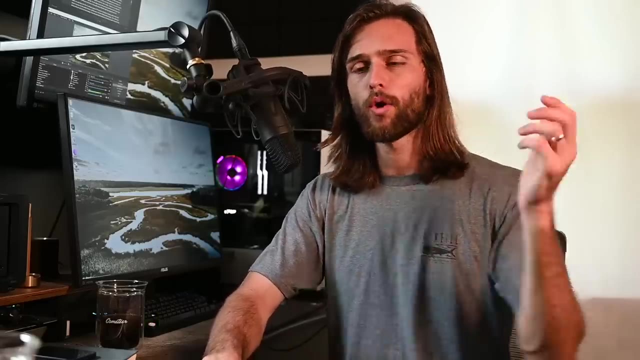 app, but solving the task at hand. Each individual task is like a new challenge for them and that is what gets them going in the morning. They know that they get to work on this task, that task and that task. They don't have to worry about the growth of the company or the growth of the app. 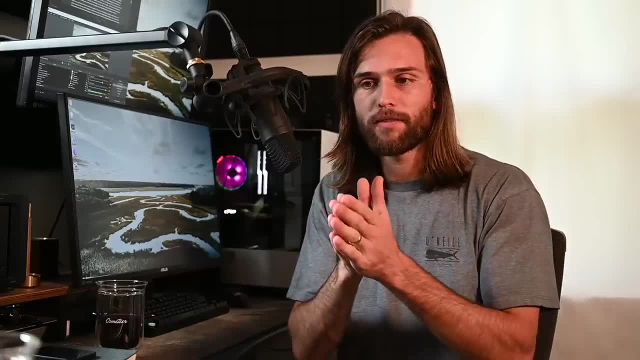 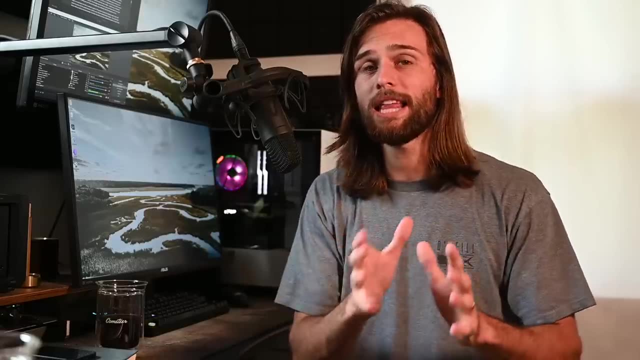 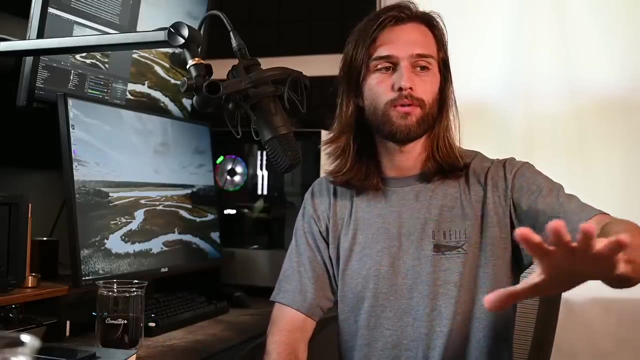 or the user interface. They are a backend developer and all they have to worry about are these tasks today, And that's basically it. There really is a luxury in that if you are wired that way, But if you are someone who got into development because you wanted to create your own apps, 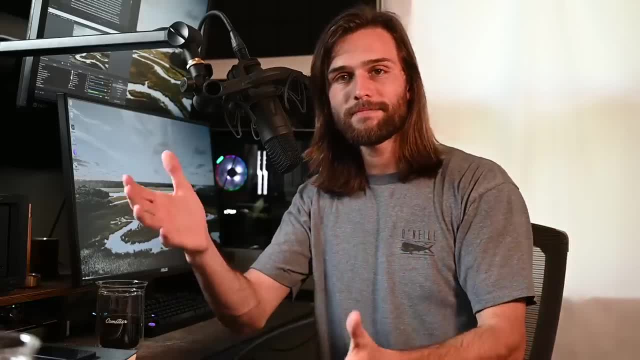 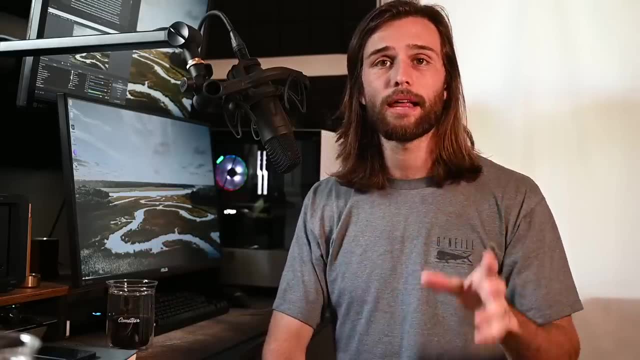 you wanted to make your ideas a reality. then it gets a little bit dicey there. But to sum it all up, many people get into coding to make their ideas a reality. It starts off as a hobby but it becomes a job once you make it your job. 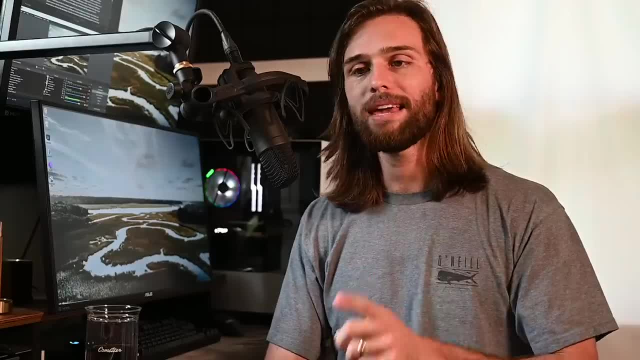 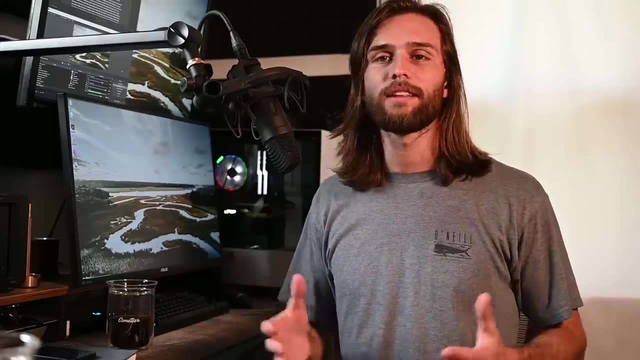 The old adage says: do what you enjoy and you'll never work a day in your life. but making something your job that you do enjoy will often times take the enjoyment out of it. So what is an actual day in the life of a software engineer? 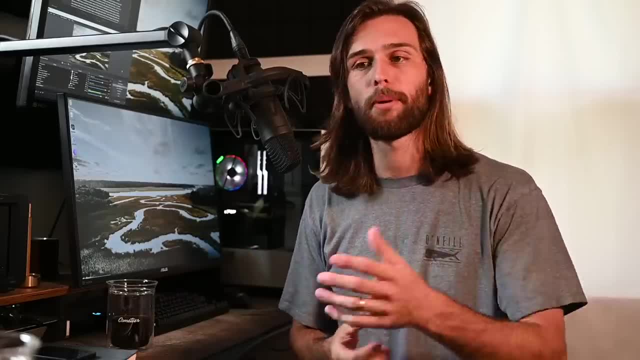 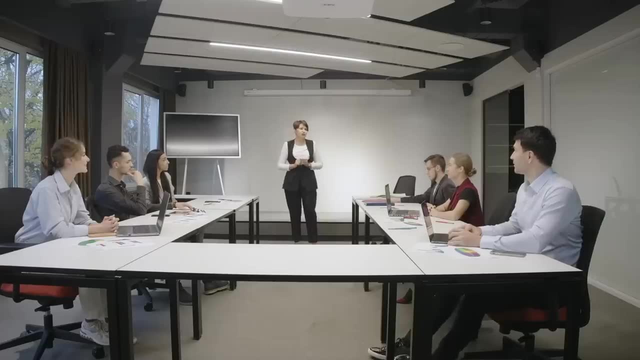 Well, this will vary from company to company, team to team, person to person, but the overall structure is typically the same. You have stand up about every day. This is when you get together with your team and you talk about what you did since the 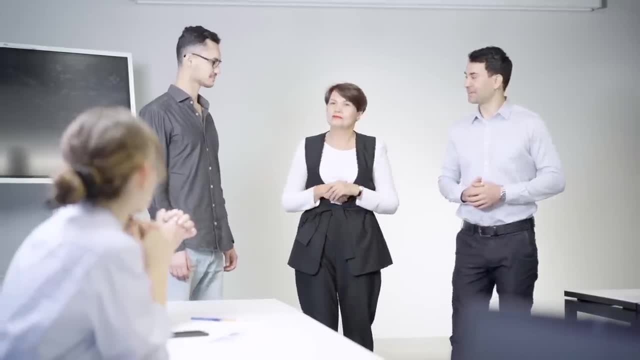 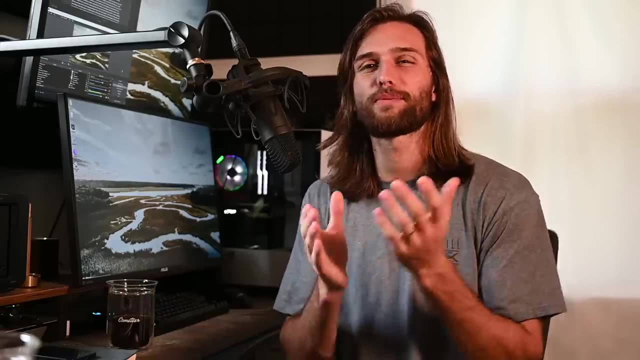 last stand up Any roadblocks that you're facing and what you plan to do next. Now, when you accomplish everything that you set out to do the day before, your confidence is through the roof. You're a genius programmer and you just want to tell everyone what you did in that stand. 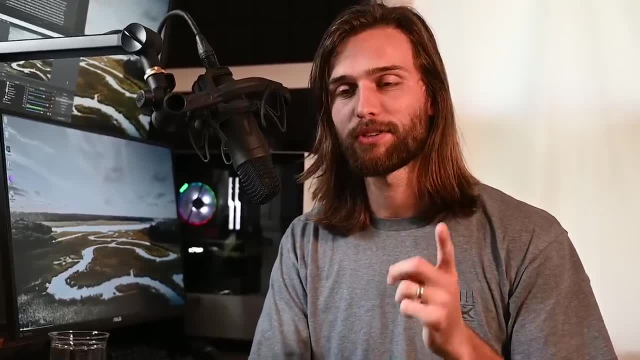 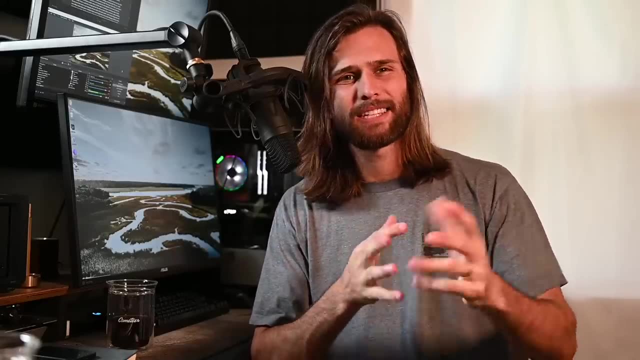 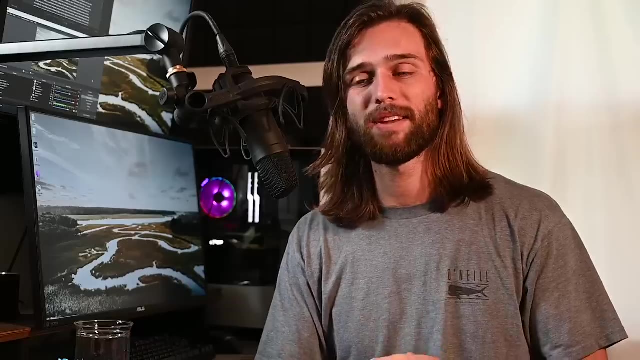 up and you love it. However, there's a flip side to this coin. If you spent the entire previous day working on a two hour task and still maybe haven't even figured it out, well then you just feel bad, Bad, Bad, No. 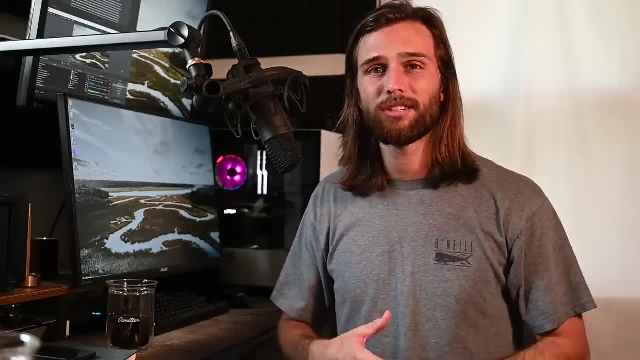 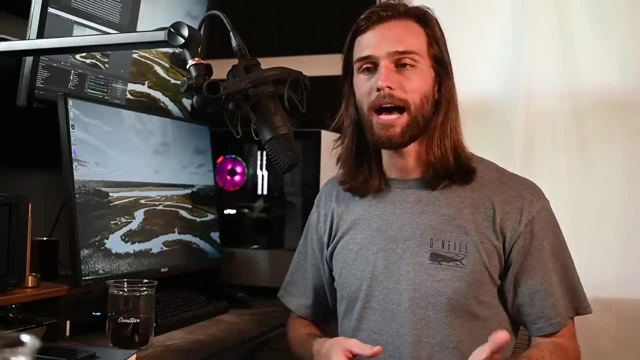 Bad doesn't really begin to describe it. You begin to maybe get a little bit anxious, You're very stressed out, You feel incompetent because you're the developer being paid to do a particular job and complete this particular task and it says it was estimated to be completed in two hours and you spent. 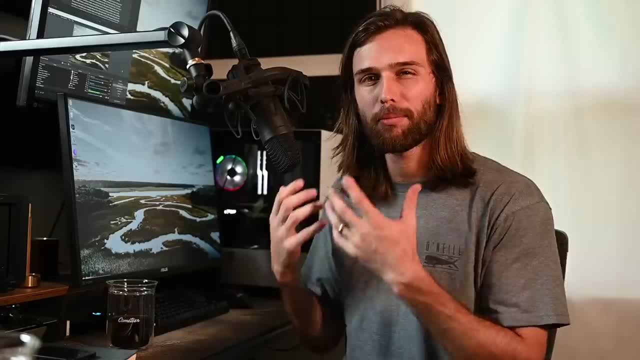 six hours doing it the day before and you still haven't even completed it. It's like if you have to present something in front of the entire class that you know you didn't do, And the whole entire class is going to be like you know what. 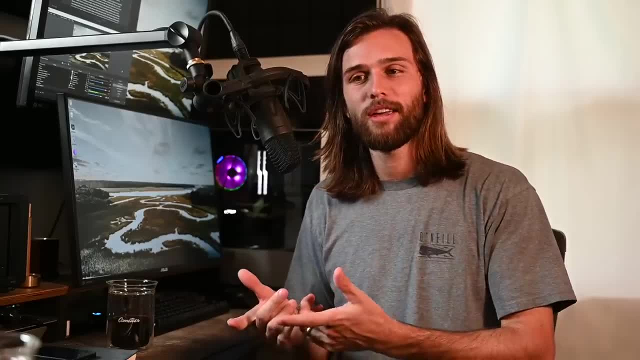 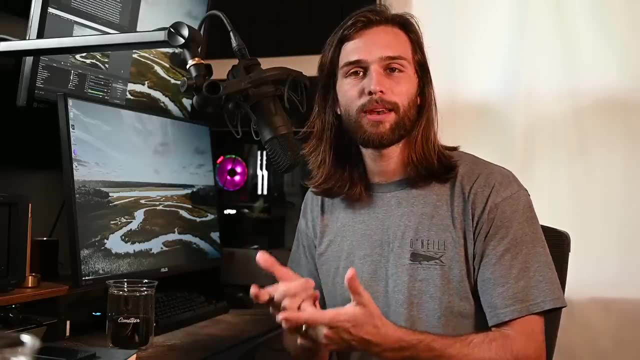 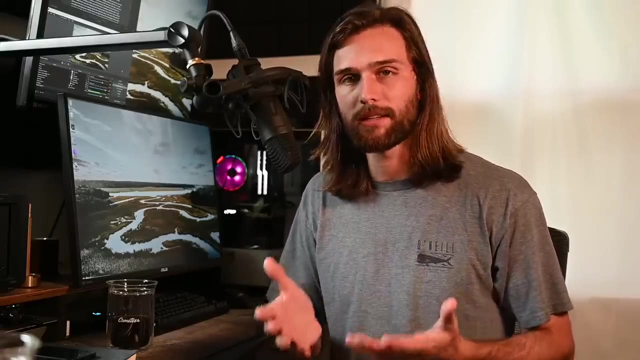 The whole entire class knows you failed. but at work you're not only worried about what your classmates think of you or your teacher thinks of you or your grade, but the stability of your job, your livelihood. I mean, you tried, but you just couldn't successfully complete the task. 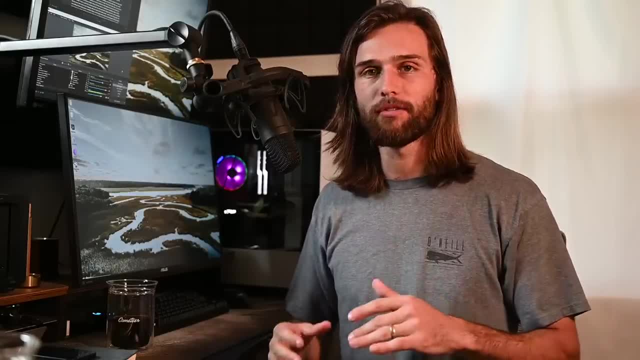 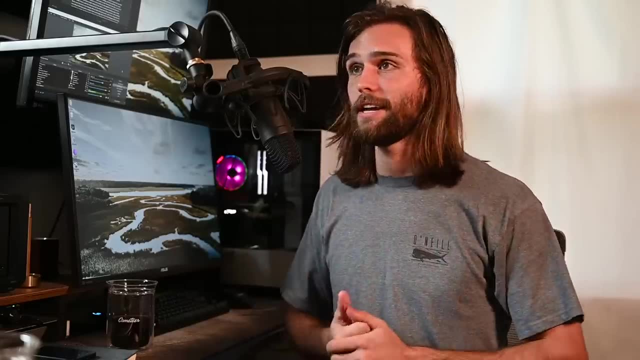 It is an incredibly stressful feeling that I hated every second of when that would happen to me and, honestly, it could just be because I felt like my team were genius programmers. I mean, in their defense They kind of were. they had 20 years experience each under their belt. 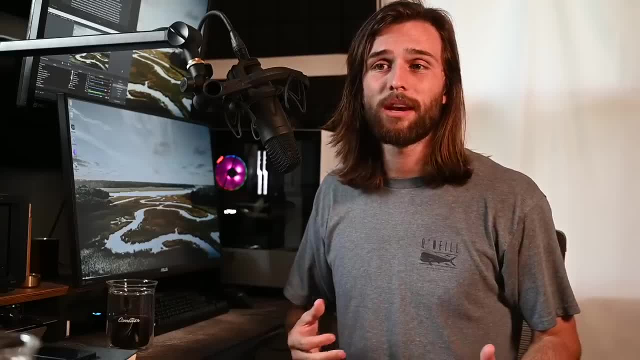 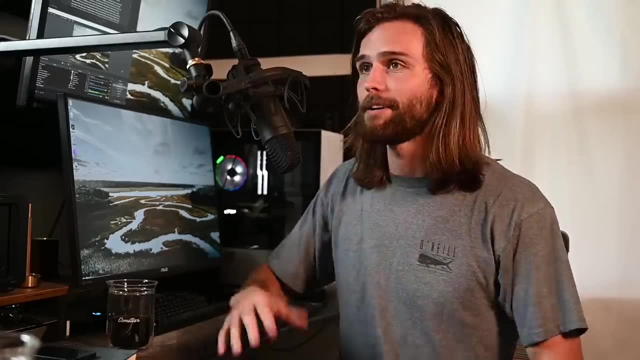 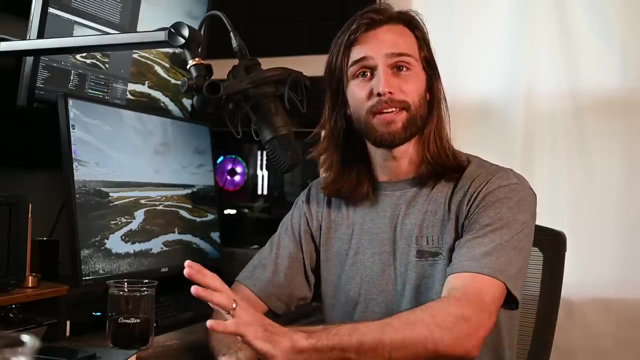 So, yeah, needless to say, I was a little bit intimidated by them, even though they were incredibly nice and helped me out. even with those traits, I still felt that way. with that being said, I can even begin to think about having a boss or a team that just like this mean or opposite of that. that would suck, but you know, maybe. 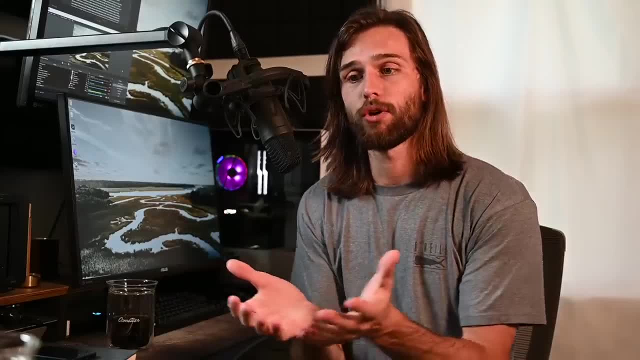 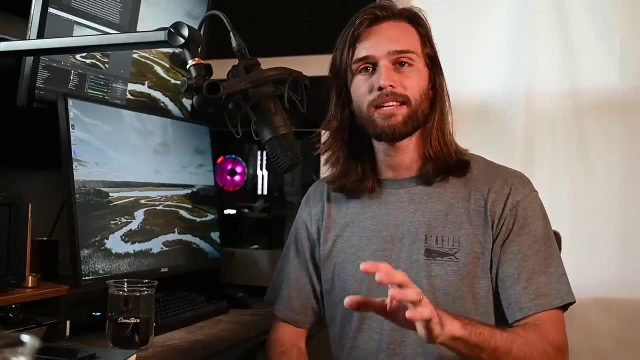 you're a better programmer than me. Maybe that stuff never happens to you, So you never have to feel that way. I don't know. I can tell you my experiences and mishaps all I want, but at the end of the day, many things cannot be learned from other people's mistakes. 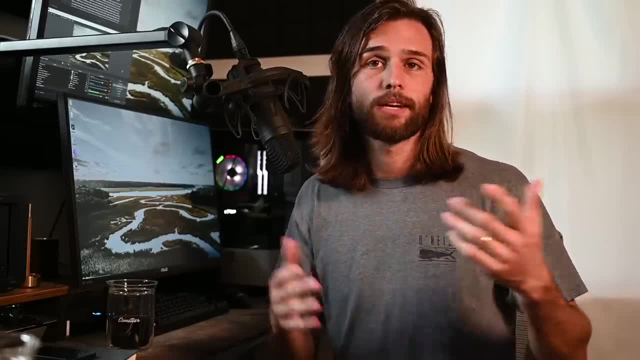 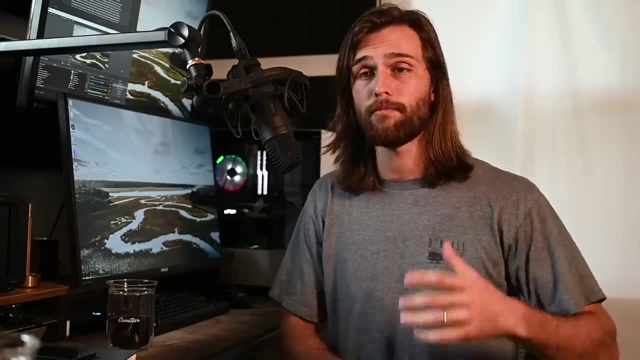 Oftentimes you have to make the mistake or, in this instance, you have to experience that situation in order to understand what it actually feels like. and maybe you thrive in those situations, Maybe you hate those situations, but you'll never know until you're in it- kind of reminds. 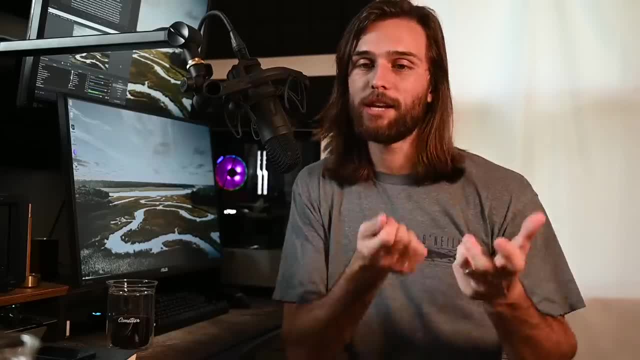 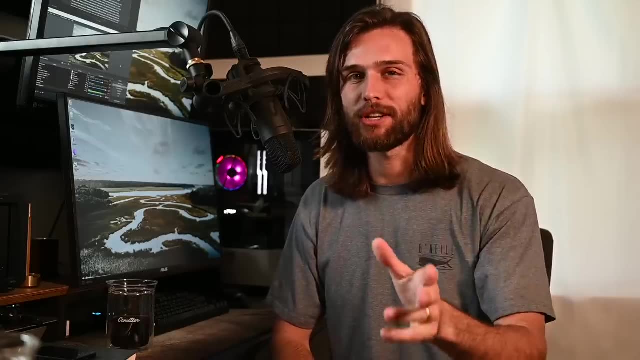 me of an analogy. It's like whenever you're at a restaurant and the waiter hands you your food, They say: oh, you know hot plate, so they put on your table, but you got to see just how hot that plate is, so you touch it. 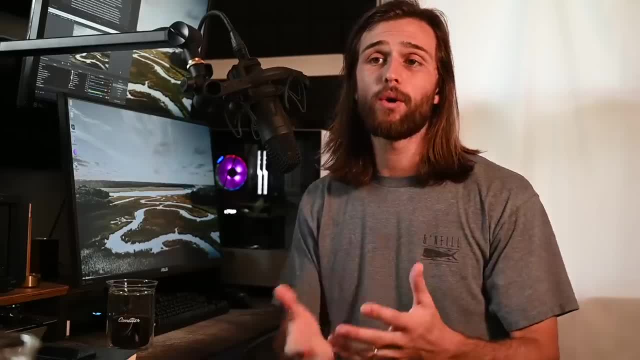 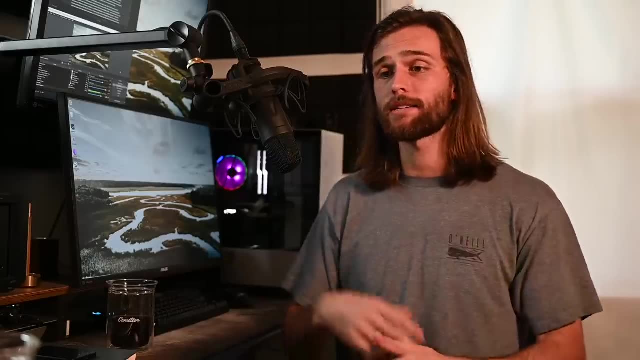 Sometimes you got to figure things out for yourself on the job. The amount of coding that is expected from you is typically around six hours. This is how they base it on tasks, So if you have a two hour task, a three hour task and one hour task, you can complete that. 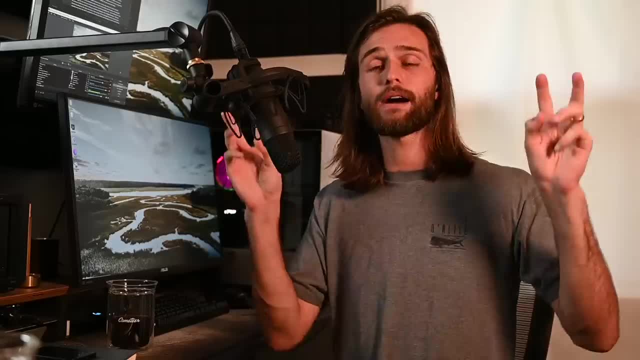 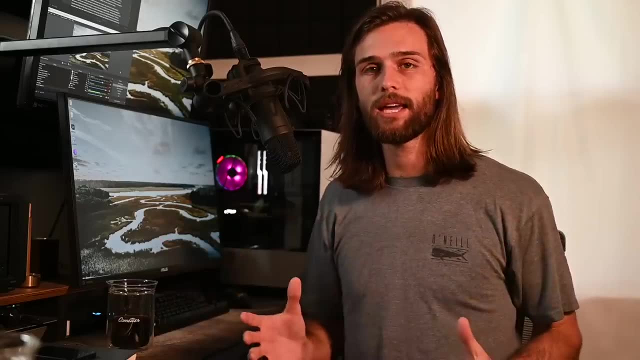 in one day, but you can't complete another two hour task on top of that for the eight hours a day, because you have stand up, You have meetings, You have breaks. All of that ties in to your eight hour day, So don't go in expecting that you're going to be coding for eight hours a day. 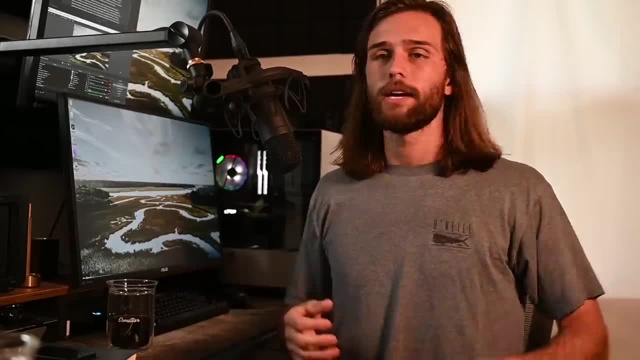 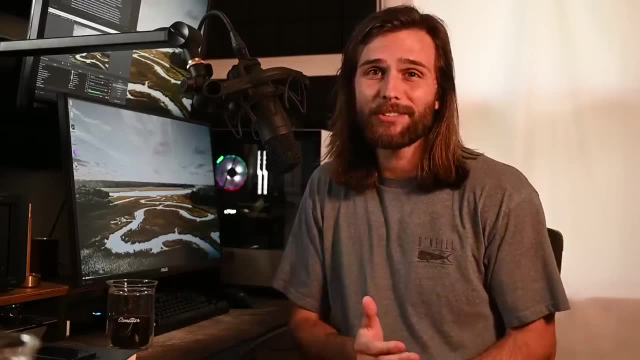 Typically, what your team should expect is around six. Now, if you've seen my video- how long I code a day- you will see that I'm typically burnout around four hours. So an extra two is a lot to handle, but it also depends on the work at hand. 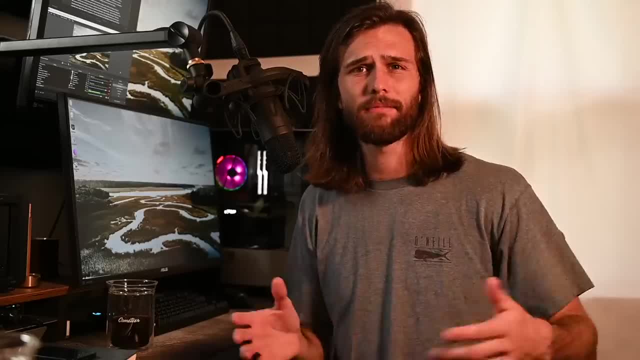 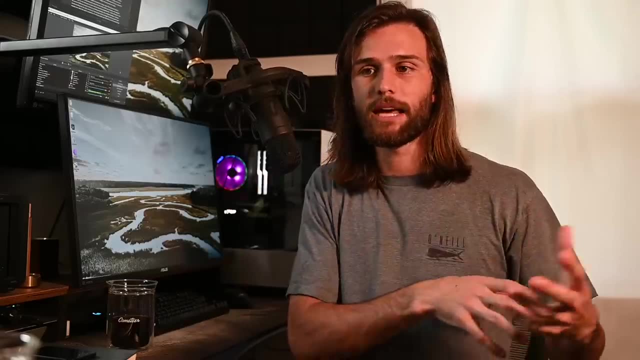 I've spent eight 10 hours almost straight. you know I have to eat and go to the bathroom And stuff, but basically almost straight coding. And when I say coding that is basically by the definition that I laid out in that video. 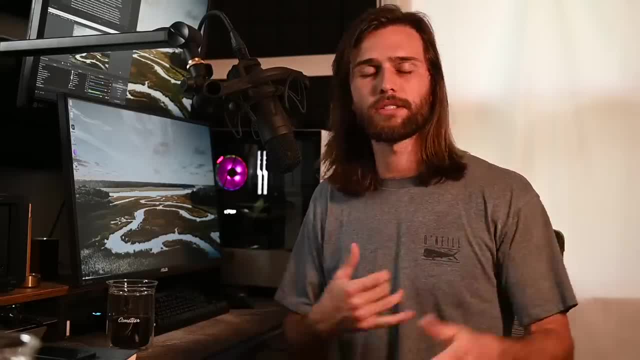 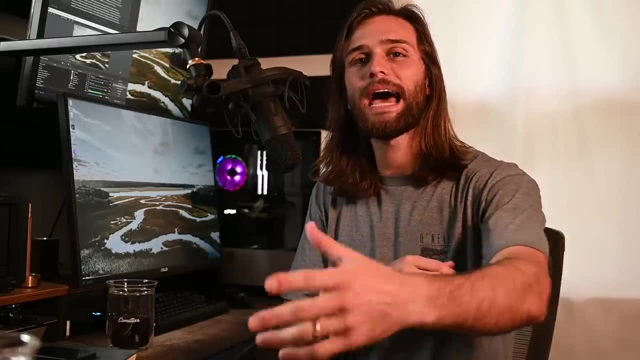 how long I code a day, and that is including everything from research to actually typing out your code. But that's when I'm working on something simple or fairly straightforward, something that's already been laid out. But when you have to figure out how to code something that has never been done in your 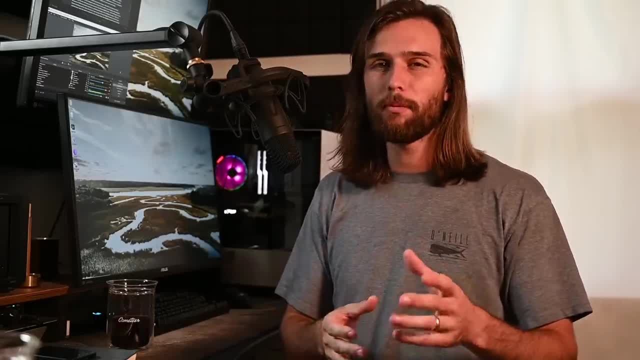 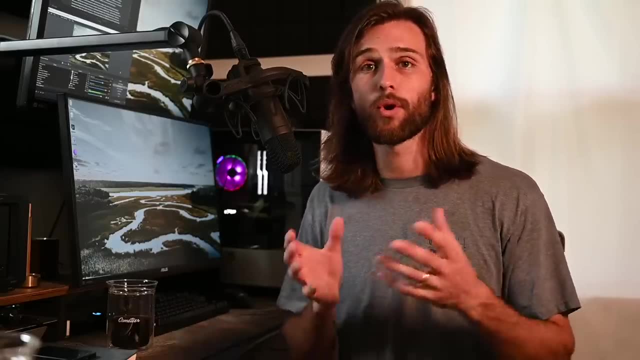 language and your stack and your context. well then, it makes things quite a bit more difficult. More brain power is needed to figure out the logic. You have to figure out how to use it In your language, with your stack, in your context, and the more brain power you use, 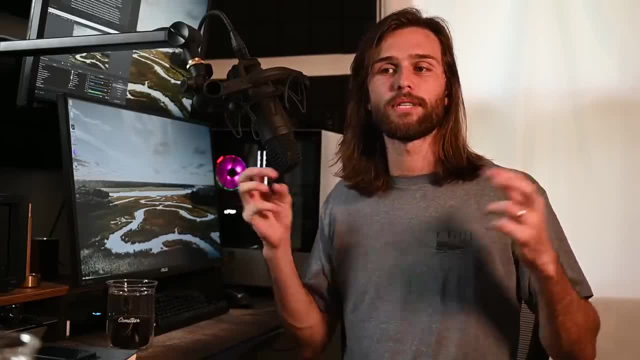 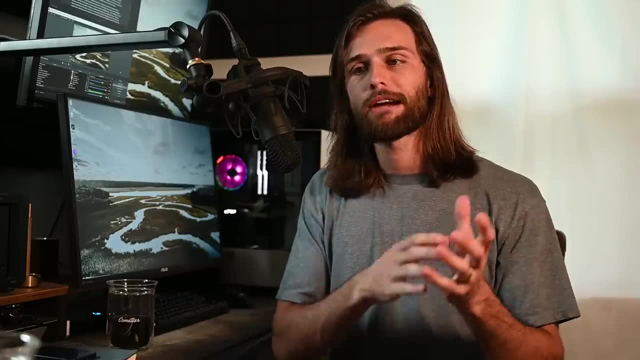 the more energy you use And the quicker you get burnt out. I don't mean burnt out and how you've been hearing it a lot lately, but just on that day. more brain power is needed to figure out the logic and to implement it in your language, using your stack and in your exact context. 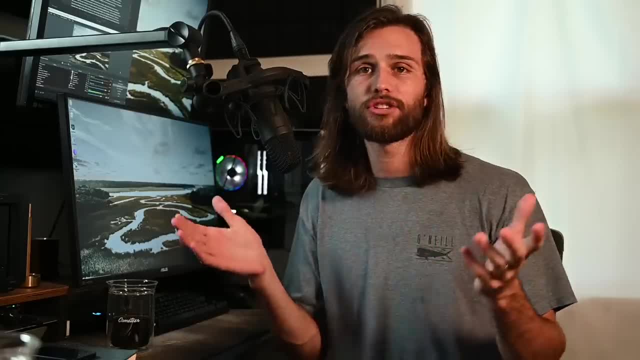 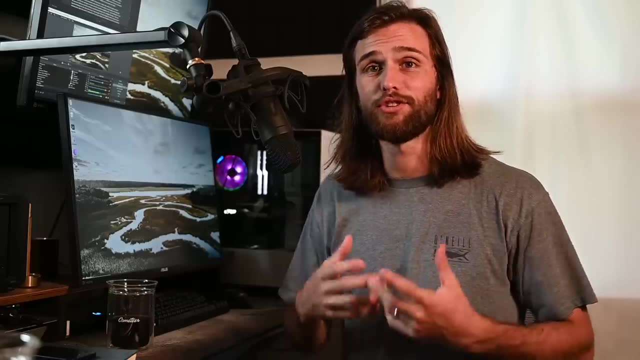 And the more brain power you use, the more drained you get and you're just tired. I've said this before: how individuals who work hard labor. We'll never understand the mental drain that it takes to do our job, because it's not physically. 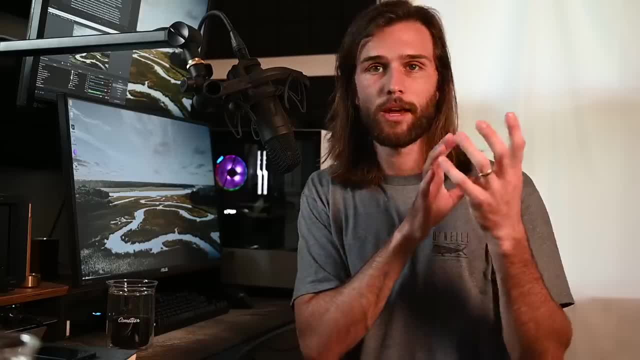 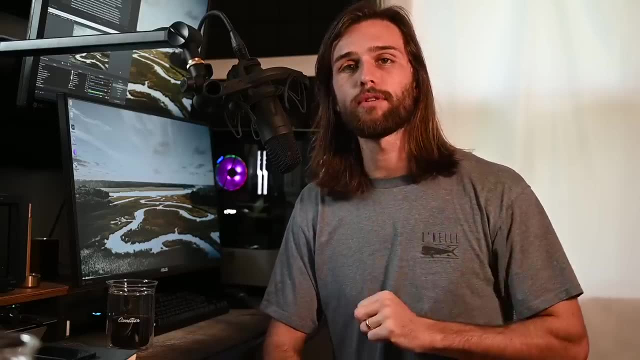 difficult And the best way I can describe the difference between those eight to 10 hour coding days and the four hour coding days. it's like digging a little hole with a little shovel for eight hours a day, compared to digging a giant hole with a real shovel. 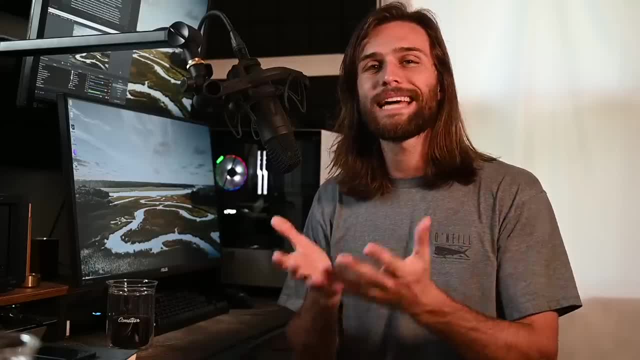 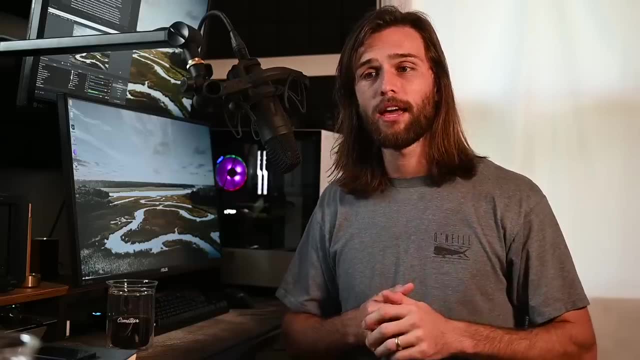 You're still digging coding, but one is much more taxing and I found to find balance of being able to figure out when I've done I've, when I'm at my wits end for that day, if I'm working on something a little bit more. 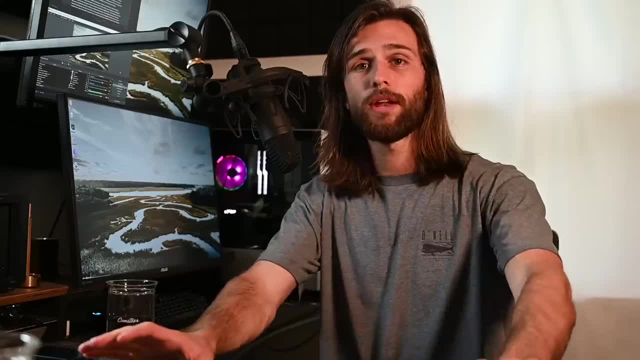 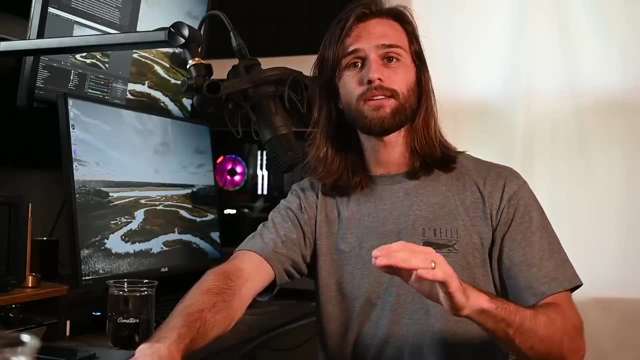 difficult than maybe. I'm in there three to four hours, don't need to worry about anything else at hand that needs to be done. I'll see that for another day. But if I want to relax and I want to do a little bit easier work, and nothing too too. 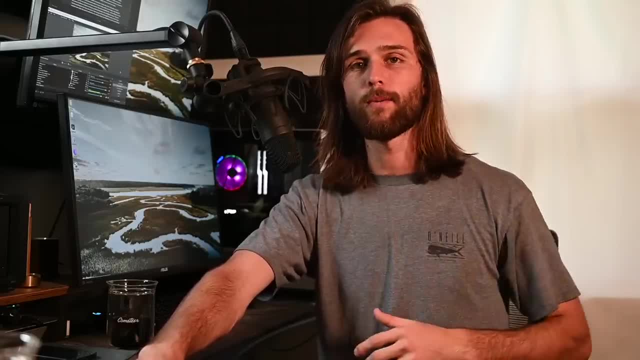 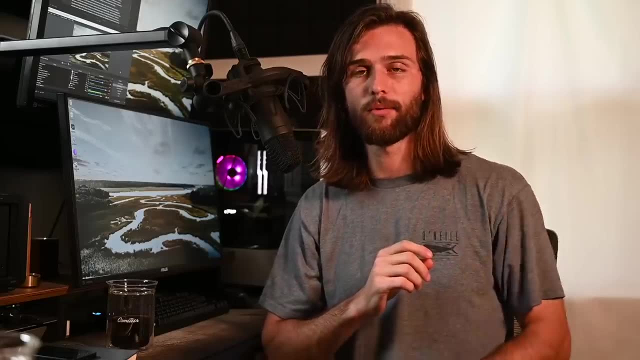 mentally draining, then I can do that too, And I can work as long as I want on my own projects. But when you're at work, you're expected to do six hours a day, give or take whatever your company wants you to do. 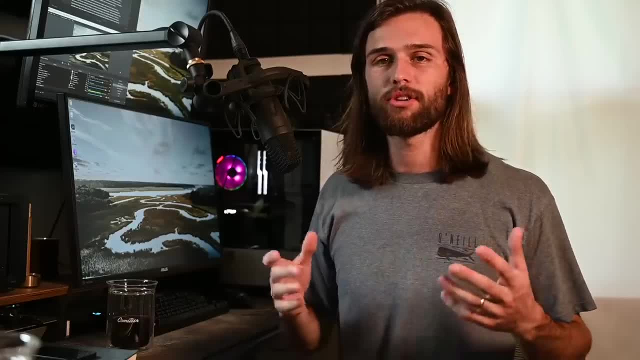 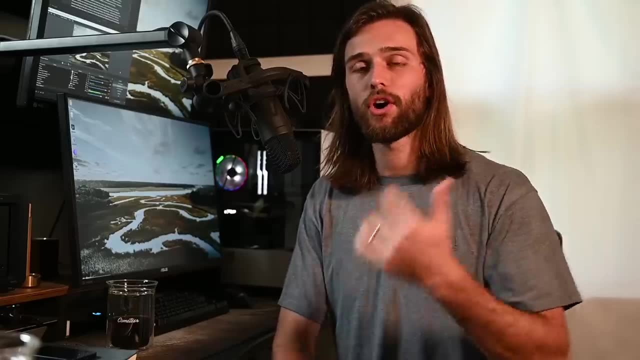 If you have to do more than the Lord, Help you. It's like all coding work is treated equally, when it's not equal. Some tasks are a lot easier than others, but if you have a lot of difficult tasks to do one day, it's hard to hit six hours of coding on difficult tasks.